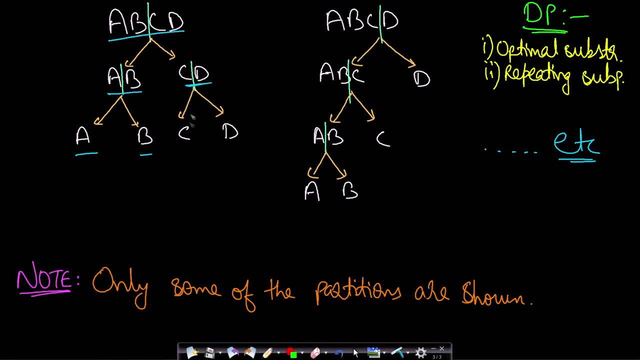 Again, we can partition it into A and B, and similarly for this C, D, we can partition it into C and D. Now, once we try for this possibility, okay for this partition. we will try for other partition points. Okay, So let's assume that we are trying for this one between C and D. 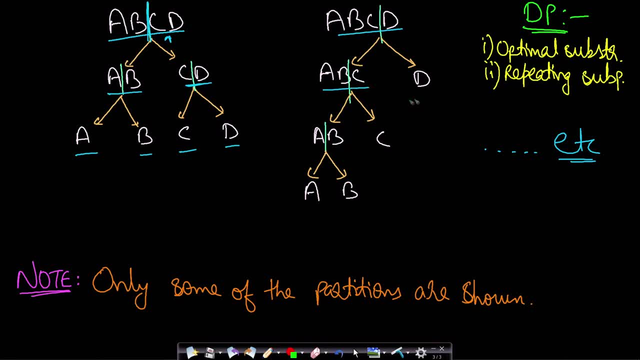 If we partition between C and D, then our sub problems will be A, B, C and D. Okay, And now again A, B and C can be divided. We can put a partition line, we can put it anywhere, But let's assume that we are putting it between B and C, So we can again partition it into. 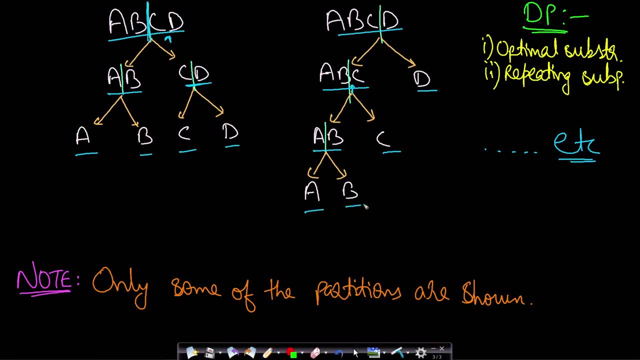 A, B and C, and again A- B can be partitioned into A and B. Okay, So you can see that this A B here and this A B here is repeating, Right? So when we are given matrices, let's. 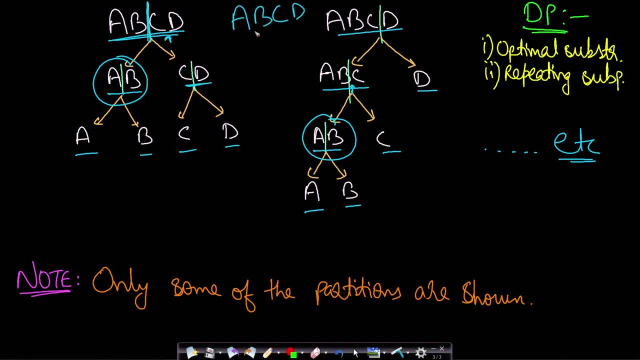 assume that we are given matrix A, B, C, D. Okay, So let's assume that we are given matrices A, B, C, D, Then we will be trying to partition at all possible points. First we will try for this first point, Then we will get some answer. We will try for the second point. 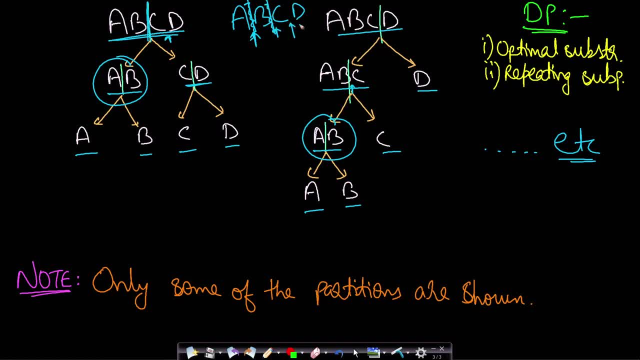 We will get some answer. Again, we will remove this. We will try. for this third point, We will get some answer. We will take the optimal out of all these possible answers. So here I have shown what will be the answer, like how the structure will look if we divide between: 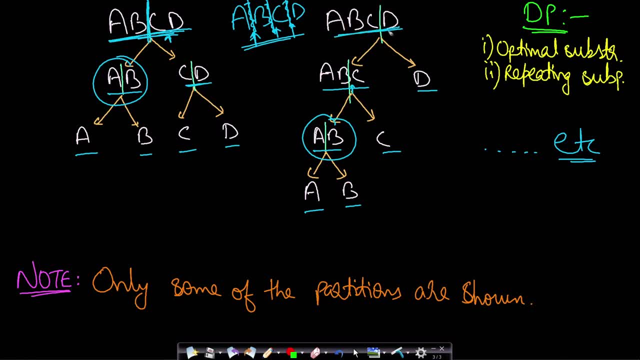 B and C. Here I have shown. if we divide between C and D, what will be the structure. Now this problem is repeating. This problem is repeating here, Okay, And this leaf nodes will always be repeating, Okay. So if you draw it completely, I have not shown the complete partitions. 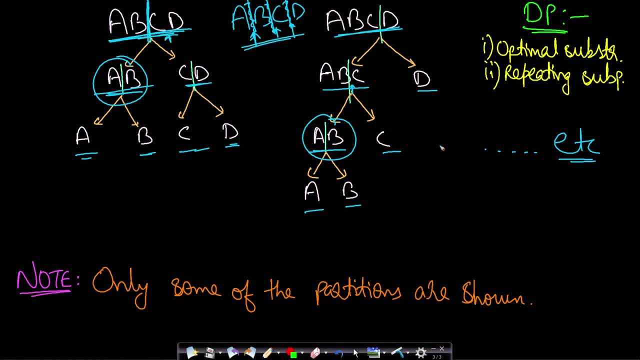 So if you draw it completely, you will find many, many repeating sub problems. Okay, So this is just to give you an idea about the repeating sub problems. Now, actually, in order to find out what will be the optimal answer, that is, minimum number of multiplications. 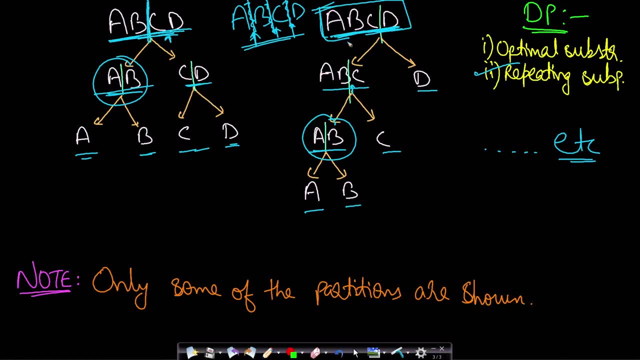 in order to multiply all these matrices, Then what we will do is we will find out what will be the minimum number of multiplications in order to form ABC and what will be the minimum number of multiplications in order to form D, And then we can find out together, by combining, what will be the minimum number. 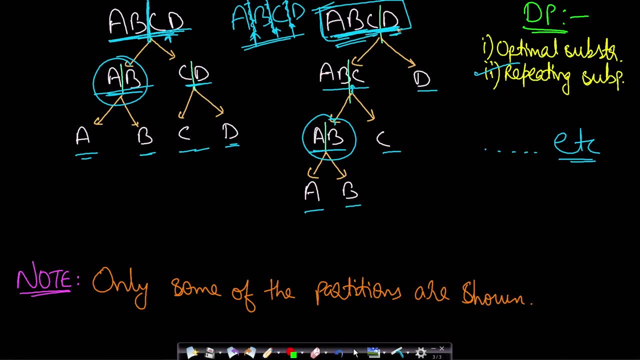 of multiplications required in order to form ABCD, provided we are dividing between C and D, Right? So what we are doing is, in order to find the answer for ABCD, we are just dividing this problem into sub problems. Okay, Dividing it into sub problems, And now we are solving these sub problems in order to 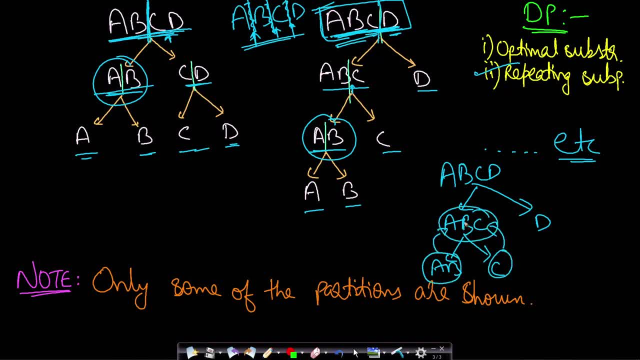 solve the bigger sub problem, Right? So, in order to solve this ABC, we need to solve AB and C. And in order to solve this ABCD, we need to solve this ABC and D, Right? So this is the optimal substructure property, which means that we can break a bigger problem. 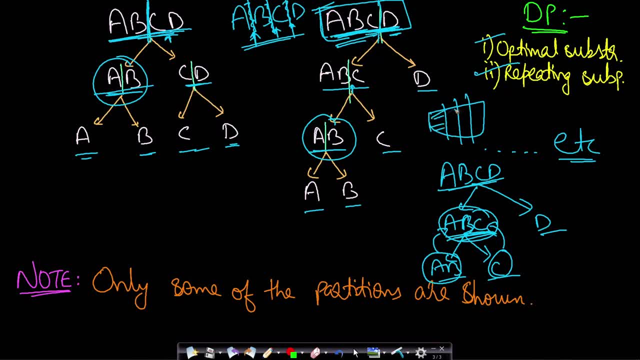 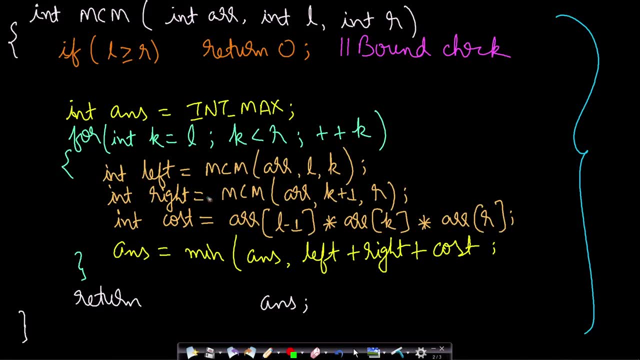 into smaller sub problems and then we can solve the smaller sub problems in order to get the solution for the bigger problem Right. So this was what we were doing in the code also, We were just partitioning using the K pointer. We were partitioning at all the possible. 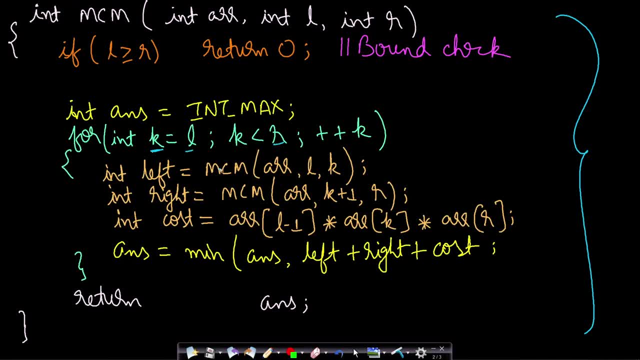 points from L to less than R, And then we were finding the answer to the left partition, we were finding the answer to the right partition and we were finding the current cost of multiplication of the two matrices, which was left and right. And then we were comparing. 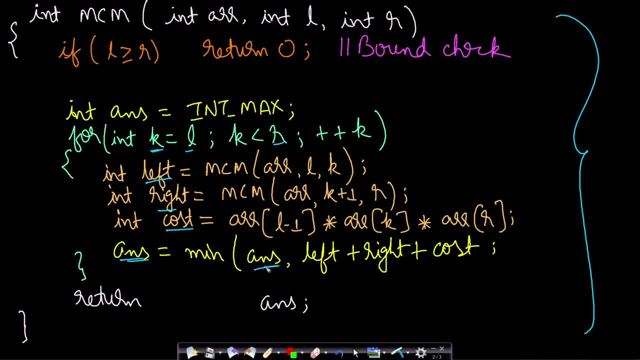 it with the answer and we were storing optimal result into our answer. Right, So this was the optimal substructure property, because we are solving the smaller sub problems, getting the answer of the smaller sub problems in order to solve the bigger problem. okay, now, this is a. 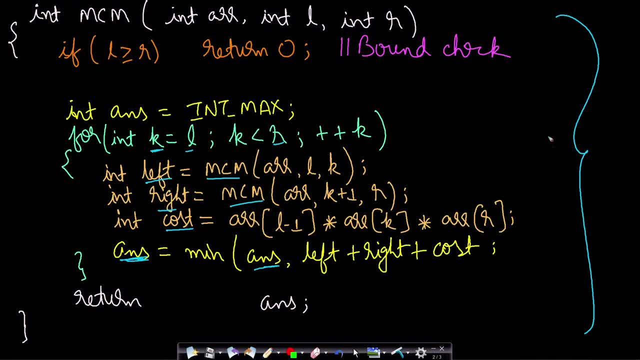 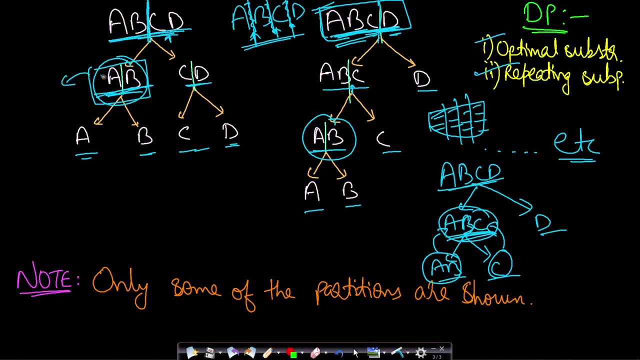 exponential time, complexity, recursive approach. now, how do we optimize it? if you can see, if we can store the result of this sub problem somehow, let's say the result is 4000. okay, if we can store this 4000, then whenever we hit this sub problem, then we can simply return 4000 without doing. 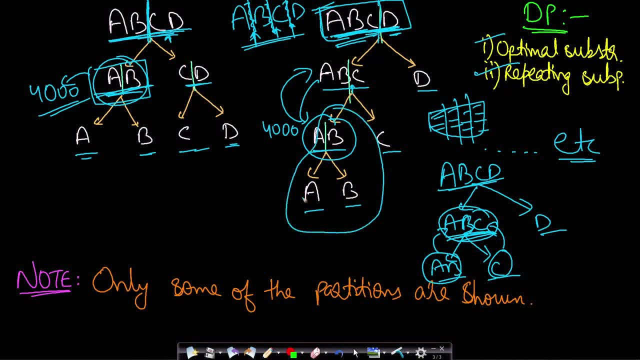 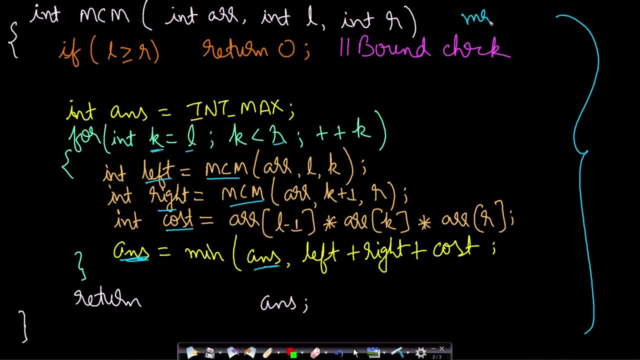 any calculation and without traversing this subtree. okay, so this will be saving us a lot of time. that is why what we can do is we can take a memoization array and what will be the size? you can take the size as n by n, okay, where n is the number of matrices you want to multiply. 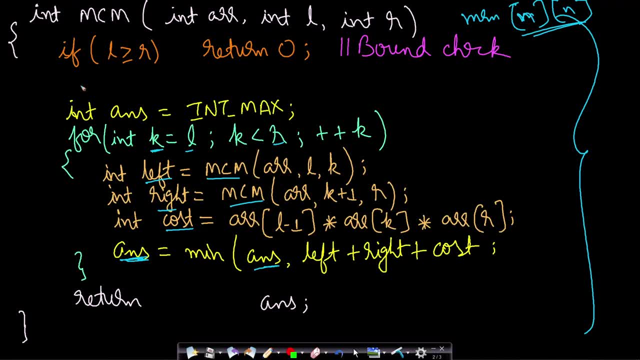 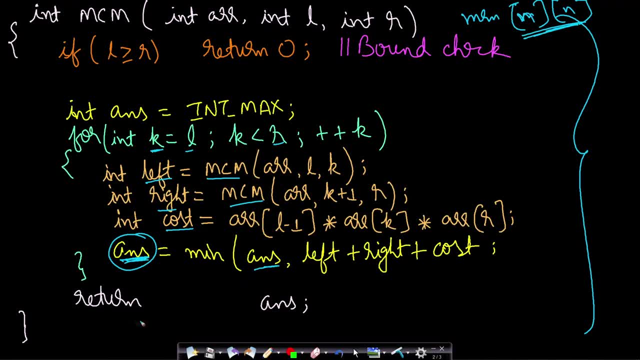 variable for this given sub problem. and now, just before returning, you want to save this answer into your memoization array so you can store at l and r, saying that the answer for partition between l to r, that means this part, will be equals to this one which is calculated already. 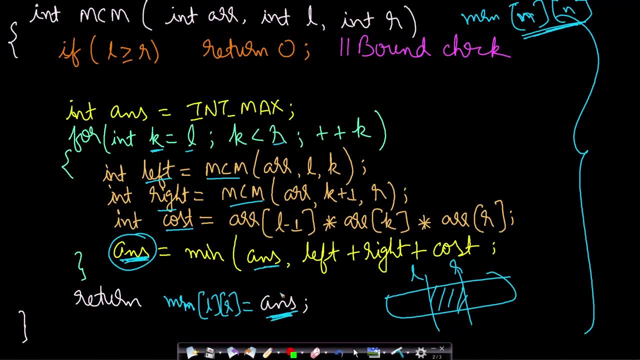 right. so the what this is doing is: this answer is getting assigned to memoization at l r, and then it is getting returned. okay, now we need to also check if the answer is already calculated, so that we don't have to perform all these calculations. so, just after checking for 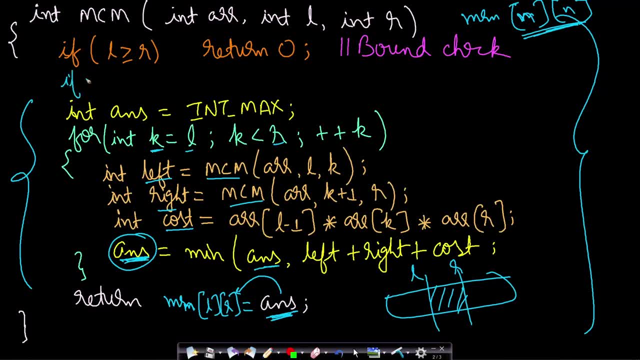 boundary check we can just insert here if memoization at l, r is not equals to, let's say, minus one, right? so what we can do is we can assign all these cells of memoization with minus one, if we know that minus one will never come in our calculation, since we are calculating the number of multiplication. 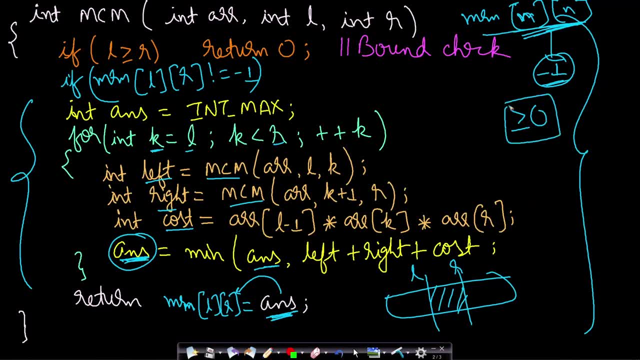 it can always be greater than equals to zero. it cannot go to negative value. so if we assign all the values of the memoization cells with a negative value, then we know that negative value can never come. and if the cell is already negative, that means it is never calculated. okay, so if 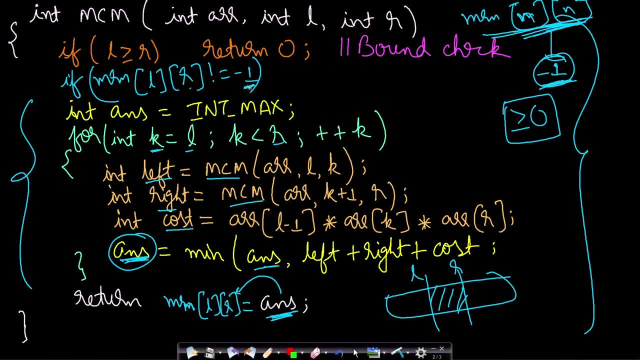 memoization at l, r not equals to minus one. that means it is a positive value. then it means that it is already calculated. so we can assign all the values of the memoization cells with a negative value and we just need to return the value at memoization at l and r. okay, so this is saving us. 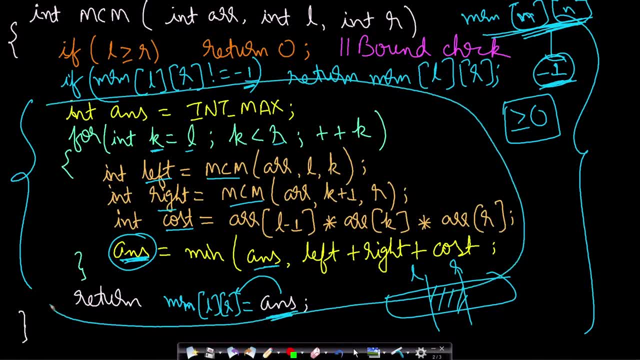 a lot of time. this entire code will not be passed again, okay, so this will save us a lot of time. the time complexity of this algorithm will approximately be order of n cube. and why it is not order of n square? because you can see here that if it was a single tree, then this: 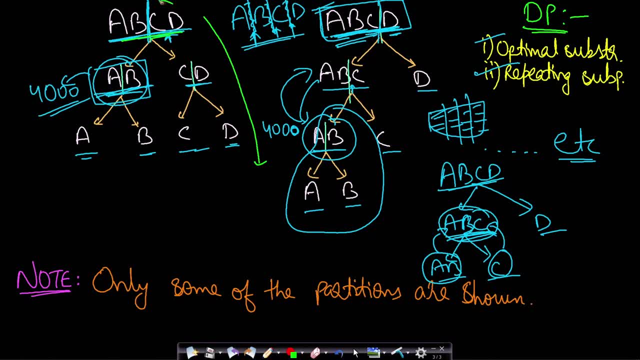 might have been order of n square, but since the root is changing n number of times, because if you are having n number of matrices, you are dividing it at n minus one number of points, so that is why we have to draw multiple trees, and that will be true for.